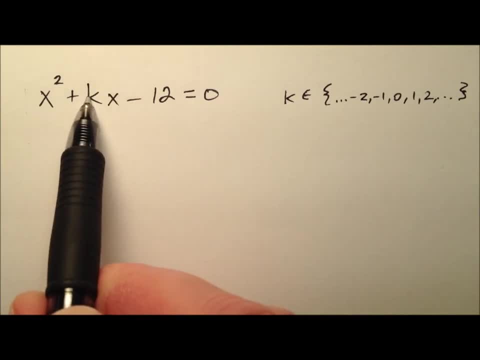 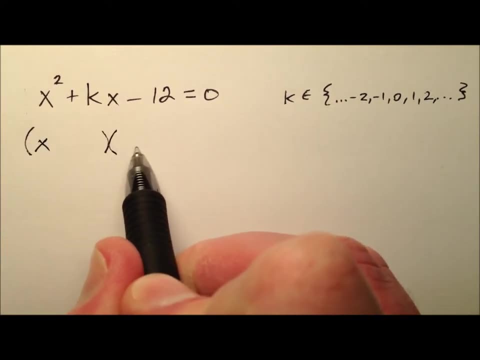 Because since k is going to be resulting in integer solutions, k itself is going to have to be an integer, which means we can factor this nicely in this form, right here. All right, and so what will go here? Well, it's going to be numbers that multiply together to make negative 12 and add to 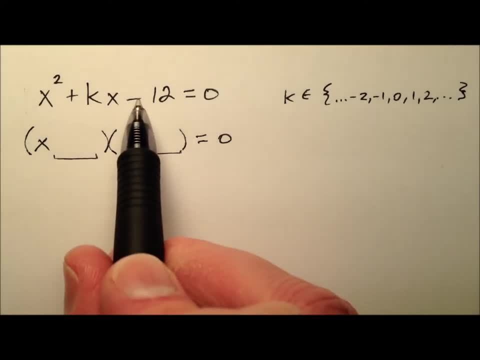 make well, this value of k, And so if we're going to multiply to make a negative 12, you know one of these factors has to be negative and one of them has to be positive, And factors of 12 are 1 and 12,. 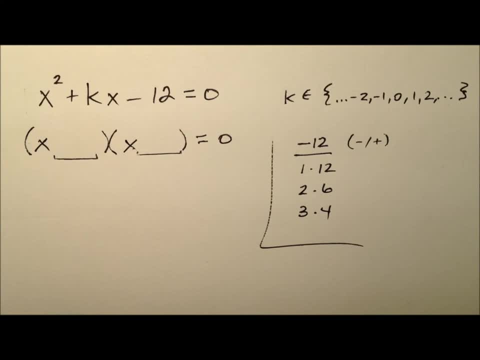 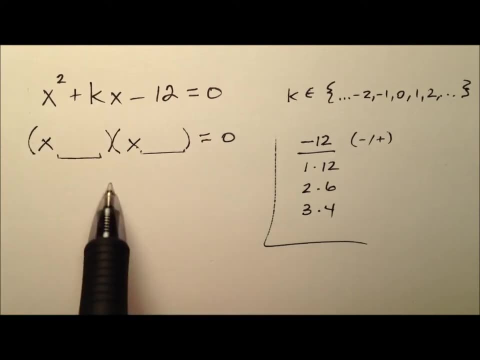 2 and 6, and 3 and 4.. Okay, so here we have laid down all the basic principles of this problem. So how are we going to go ahead and attack this? Well, if they multiply to make a negative, 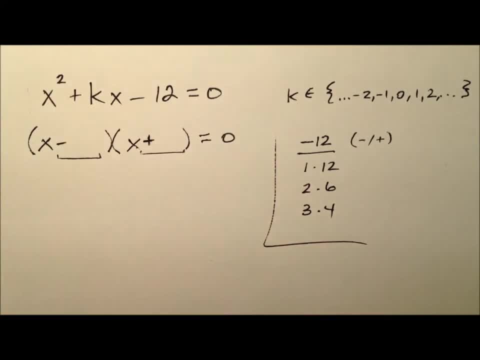 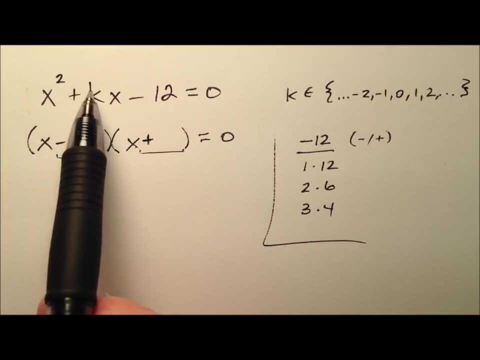 we decided that 1 is negative and 1 is positive, because that's how we multiply to make a negative, All right, and they add to make. well, it doesn't really matter if it's positive or negative, because k could be positive or k could be negative. We're just saying plus kx. 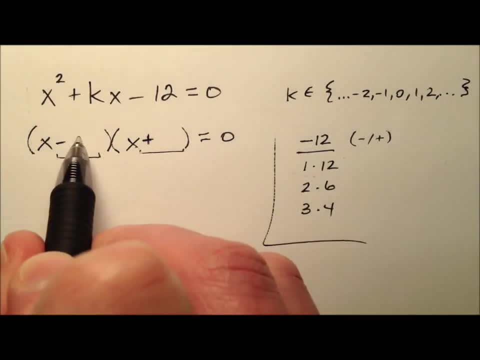 Okay. so let's go ahead and look at this 1 and 12 first, And let's just go ahead and put 1 here and 12 here and just see what happens. So when I multiply this out, I'm going to end up with: 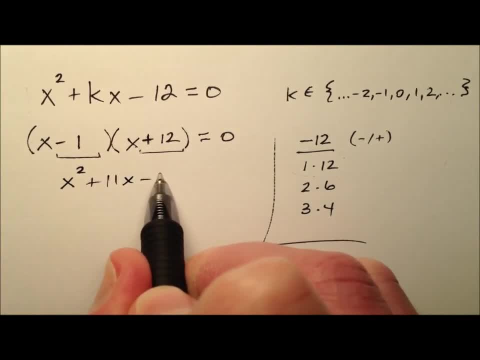 x squared plus 11x minus 12 equals 0.. So, in this case, my solutions, well based on this factorization, will be: x equals 1.. negative 12,, which are integer solutions, and my value of k will be positive 11.. 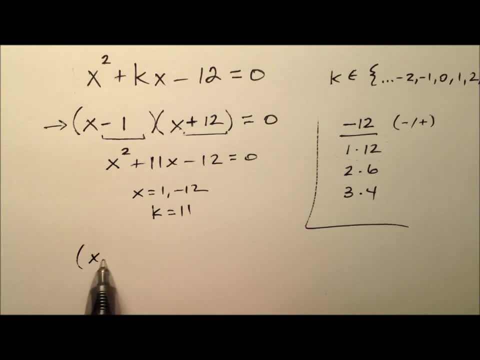 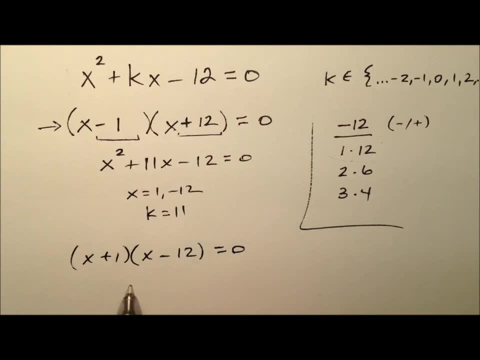 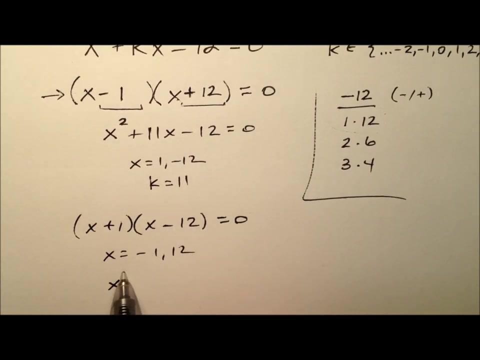 All right. well, what if I had switched these up? And what if I had said: x plus 1 and x minus 12 equals 0, essentially just changing the signs? Well, my solutions are negative: 1 and 12, again integer solutions. And when I multiply it out, x squared minus 11x minus 12 equals 0.. 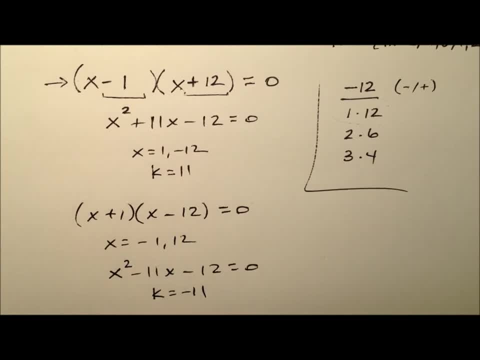 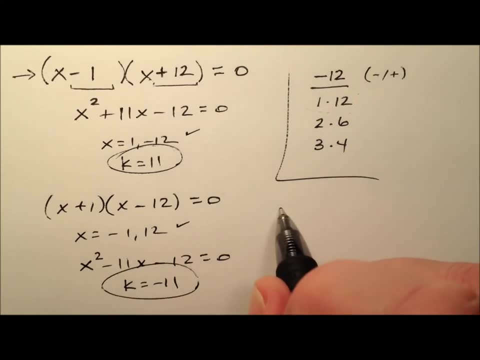 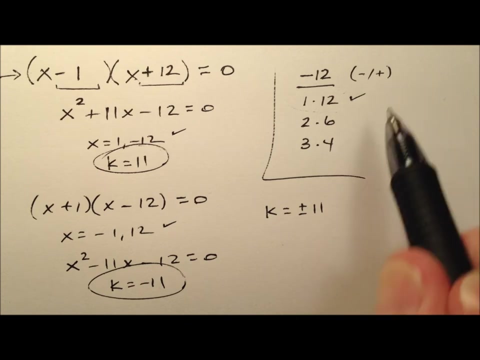 And so here we see, our value of k is negative 11.. So integer solutions positive 11.. Integer solutions negative 11.. All right, so it seems like k can equal plus or minus 11, just for starters. And that's when we consider the factor pair 1 and 12.. Well, using 1 and 12, where did this 11? 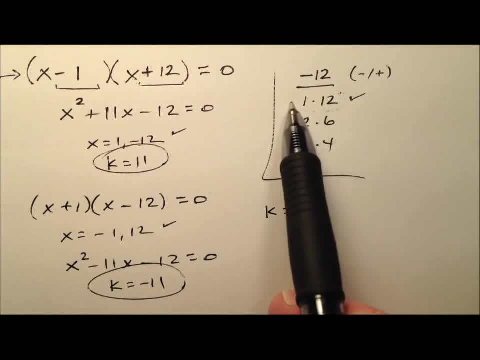 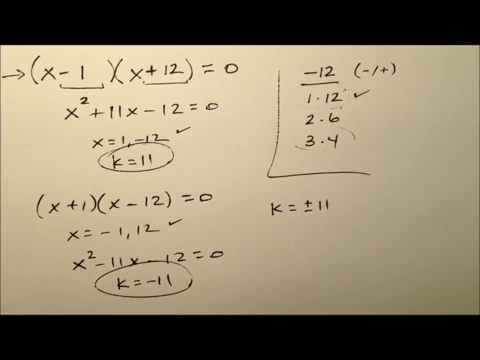 come from? Well, because 11 is the difference between these two factors. 12 minus 1 is 11.. Well, I wonder if that will. we'll follow with my 2 and 6 and my 3 and 4.. And so let's go ahead and look at those. So x minus 2. 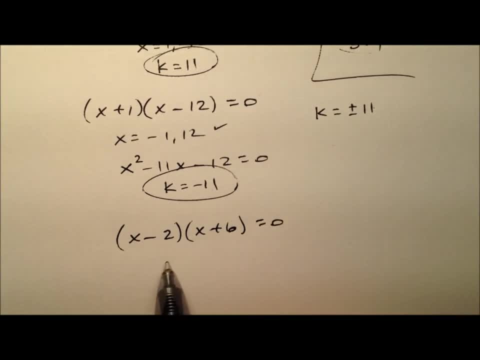 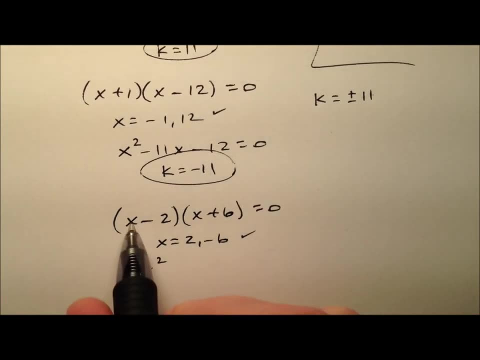 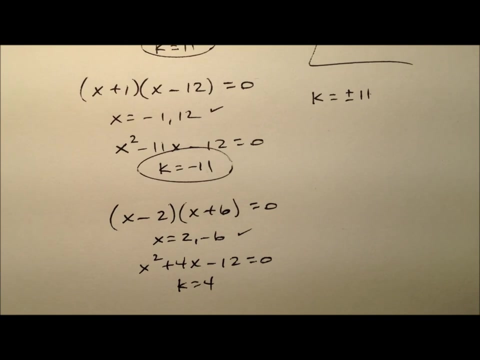 and x plus 6.. This will give me positive 2 and negative 6 for solutions which are integer solutions, And when I multiply it out it's going to be x squared plus 4x minus 12 equals 0. So that value of k is 4.. Once again, 4 is the difference here, And so if we were to switch, 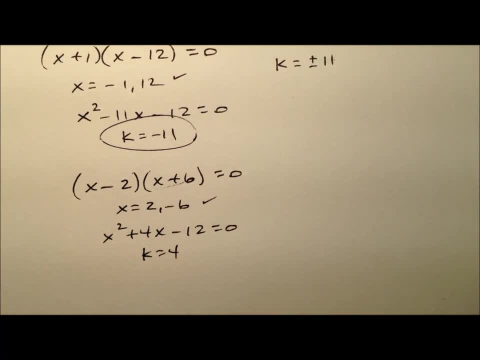 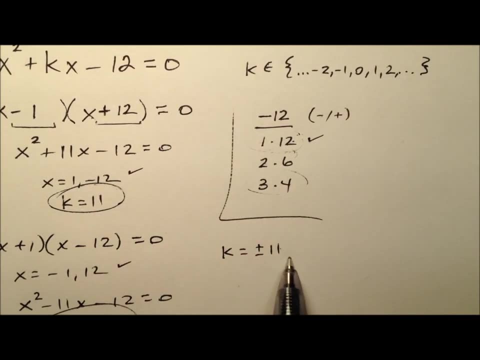 these up, we would end up with k equals negative 4 as well. So we can go ahead and kind of follow that approach. and so, based on the factors 1 and 12, we get k equals plus or minus 11.. From the factor pair 2 and 6 we'll get k is plus or minus 4, and then from the factor pair 3 and 4 we'll get: 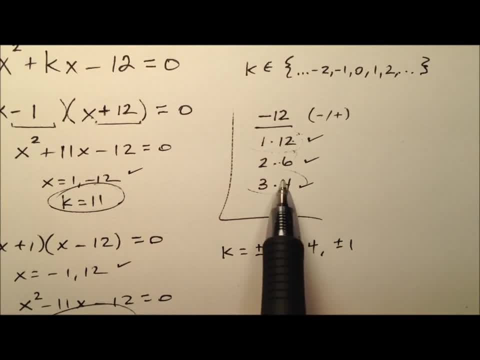 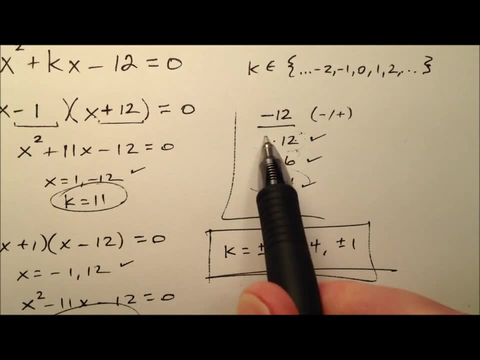 k equals plus or minus 1, because 4 minus 3 is 1.. So I know that these are all the possible values of k, because these factor pairs are all the possible factor pairs for 12, using whole numbers, that will result in integer solutions. And so, to answer this question, what values of k? 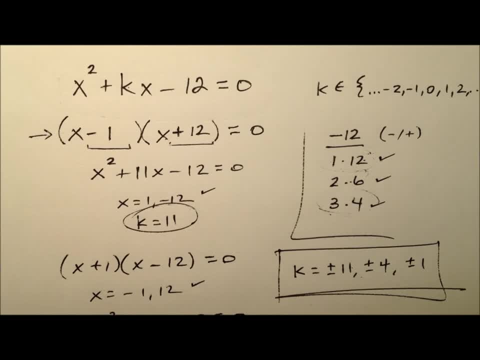 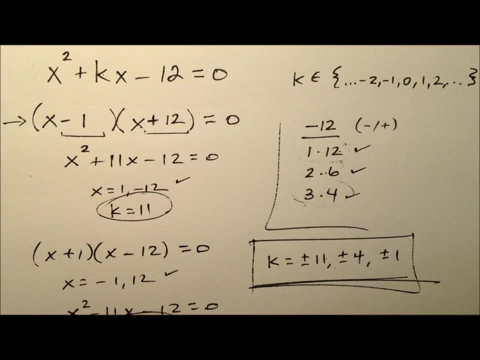 will give me integer solutions when I solve this for x. Well, I'll have six values of k, of K. K equals plus or minus 11,, plus or minus 4, and plus or minus 1..